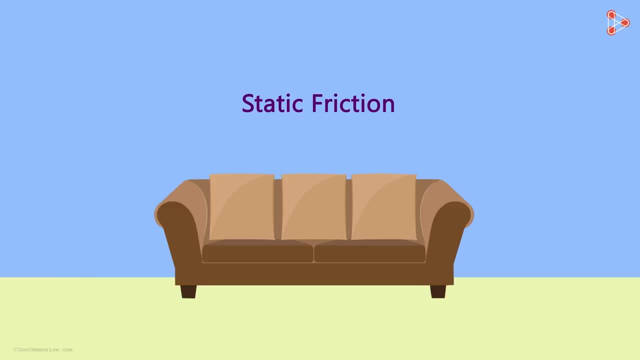 Well, the answer is static friction. The force that you apply is balanced by a frictional force, by the floor, And this force is applied in the direction opposite to your push. This force is nothing but static friction. The concept of static friction is really amazing. 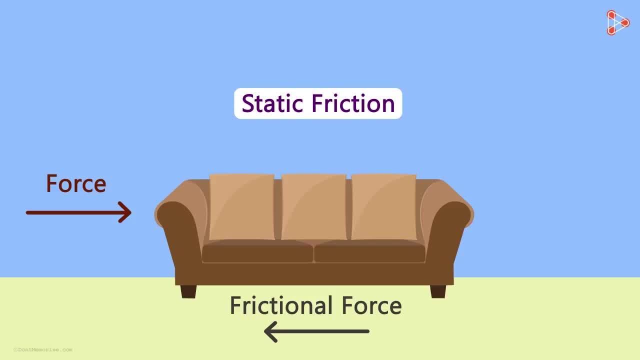 Why do I say that? The reason why I say that is because it is a self-adjusting force. As you increase your force of push, the force of static friction increases too, and the forces are still balanced. Now I know what you must be thinking. 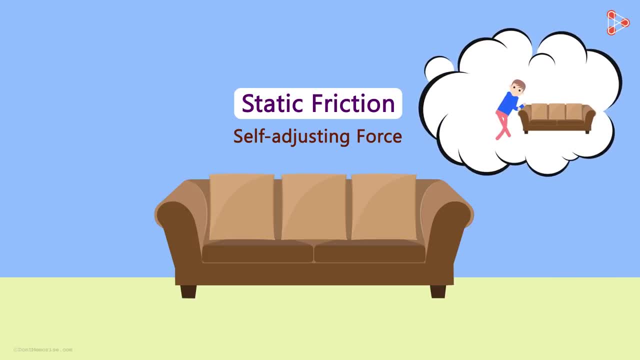 After a few seconds, the sofa begins to move right. What happens to the static force then? Let's discuss this with the help of a simple graph. We assume that the force you apply is a horizontal force, represented by the X-axis, And the force is a horizontal force represented by the X-axis. 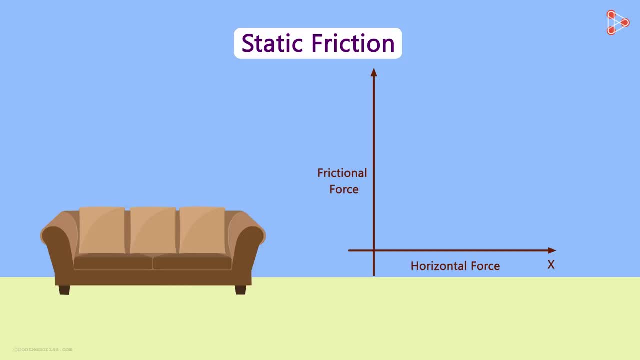 And we assume that the force you apply is a horizontal force, represented by the X-axis. The frictional force applied by the floor is represented by the Y axis. Now, as you increase the horizontal force applied, the frictional force is also increasing accordingly. to keep the sofa at rest. 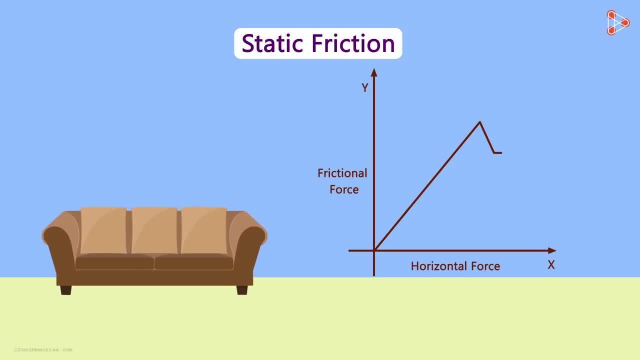 This continues till a point where the sofa just starts moving And that's where the static friction ends and the sliding friction begins. The sliding friction is more or less constant. if you notice, This part of the graph is static friction. It's when the sofa is not moving in spite of the force you're applying. 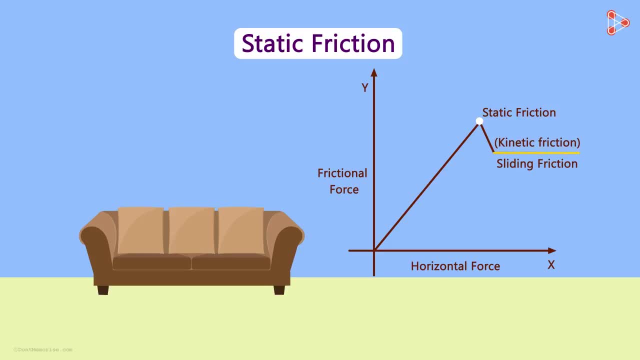 And this part of the graph is sliding- or kinetic friction. when the sofa begins to move, The point around which the sofa just begins the movement is called the breakaway point. Is there anything else you noticed in the graph? Why is this line at a lower level than the maximum static frictional force? 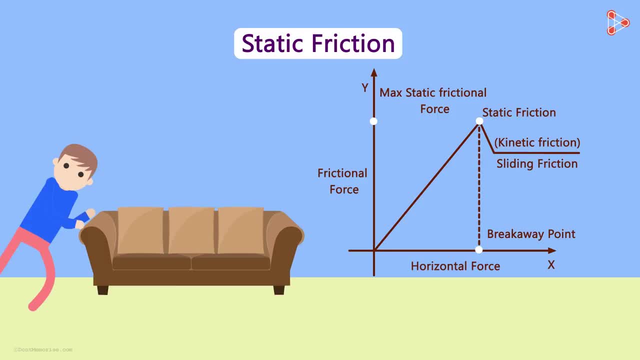 The reason is simple. If you have ever pushed a sofa or some heavy object on the floor, you would have realised that pushing it is a little easier when it's in motion. Yes, it's because the sliding friction is lesser than the static friction that's offered.